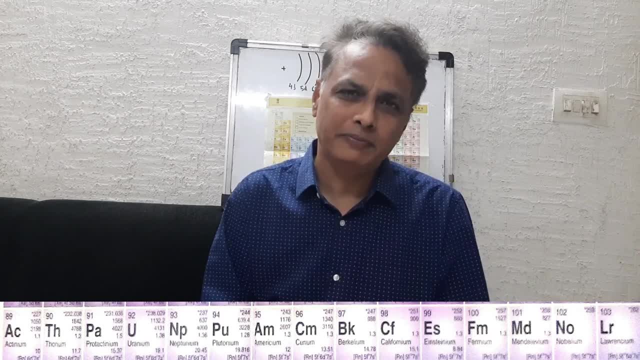 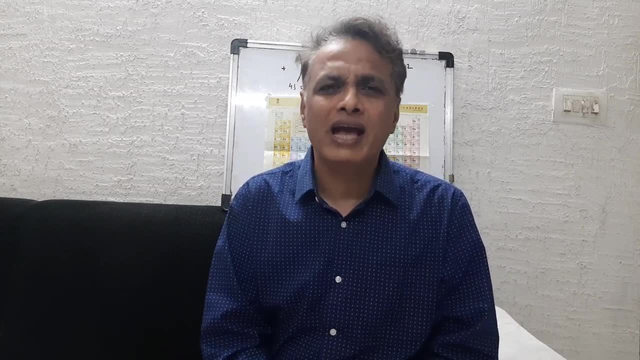 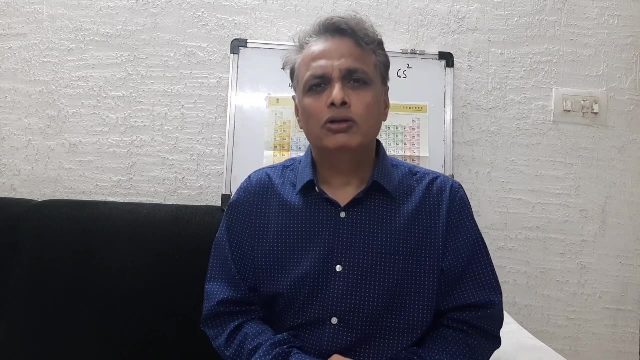 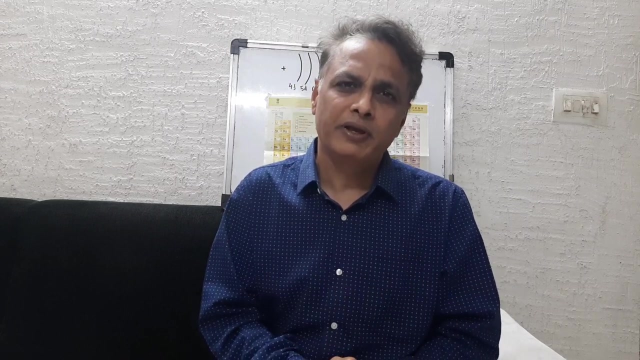 orbital are known as fire block element. this for a block element or lengthen and elements are also known as a rare earth element. why this is known as a rare earth element? why this is known as a rare earth element? because these elements are obtained from minerals present in the soil and their 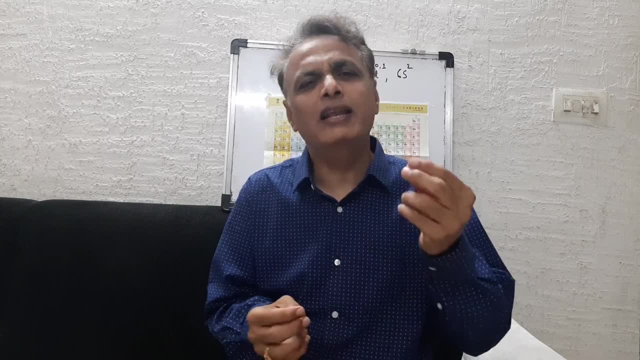 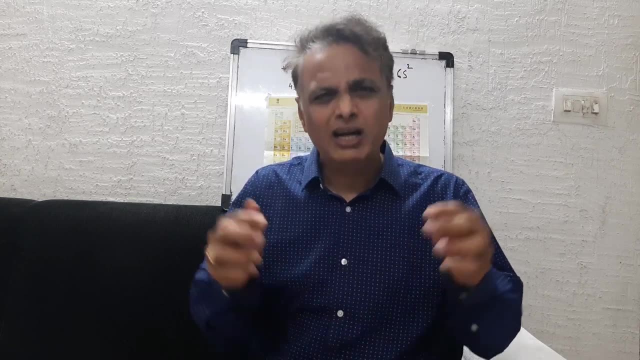 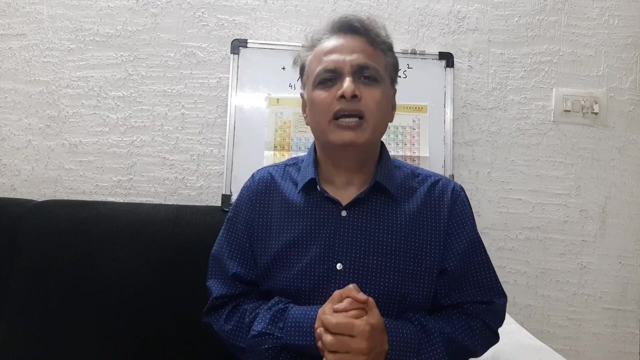 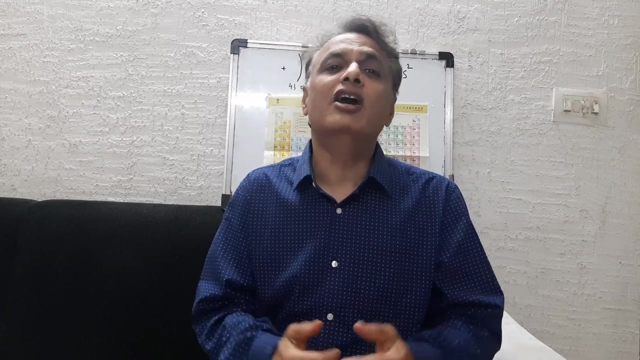 quantity in the soil or mineral is very less and therefore they are known as rare earth element, but nowadays this word is not appropriate because most of the element are obtained in large quantity. these elements are also known as in a transition element. these elements are also known as in a. 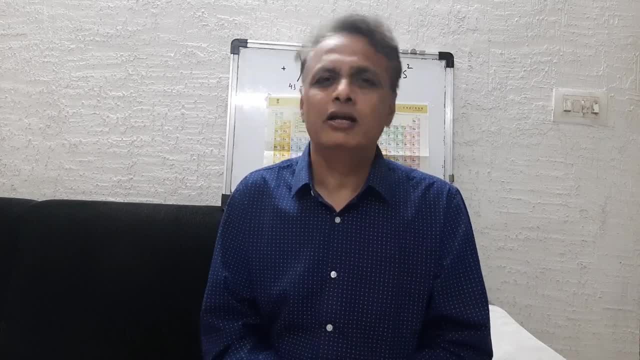 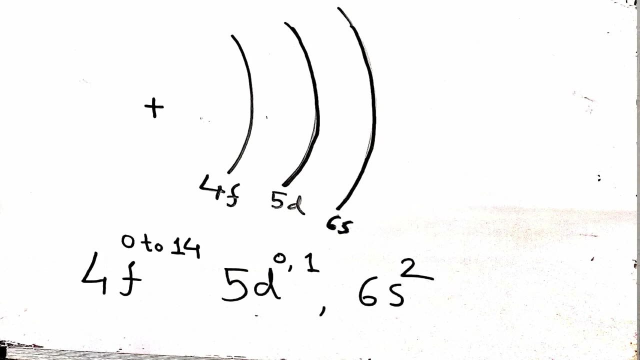 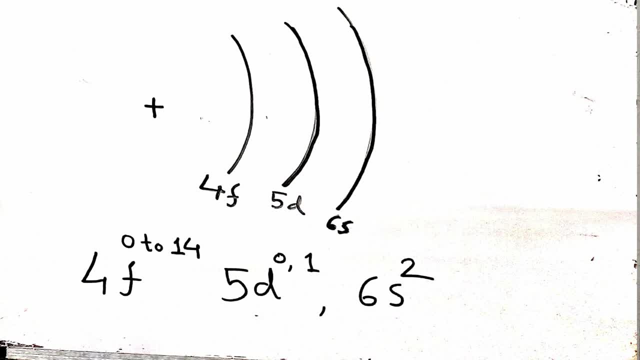 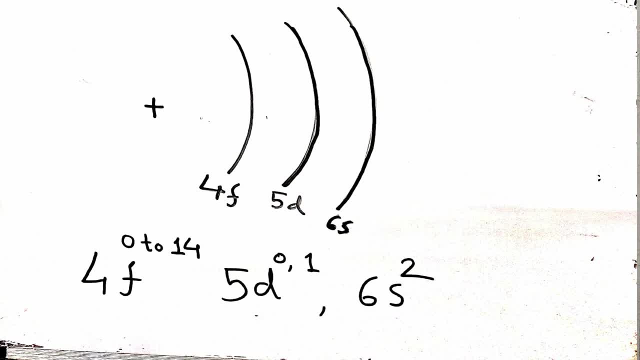 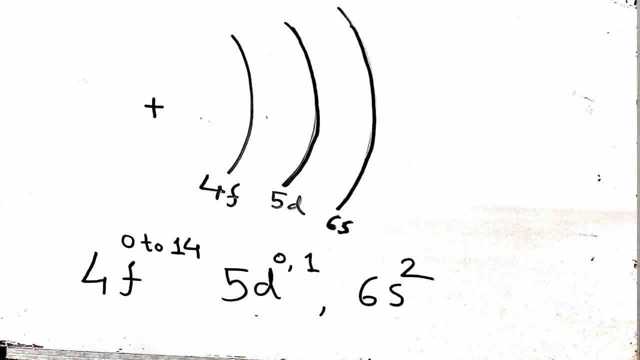 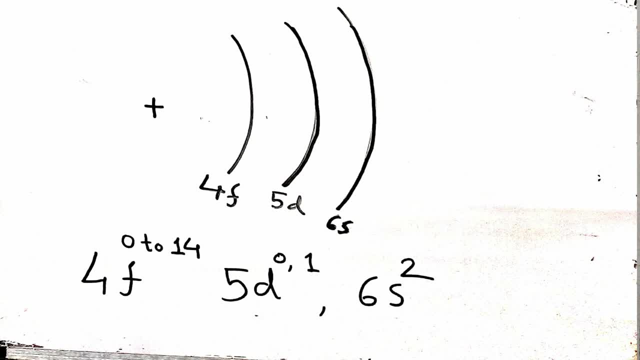 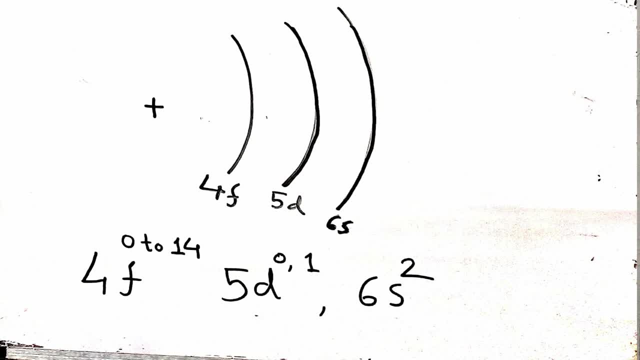 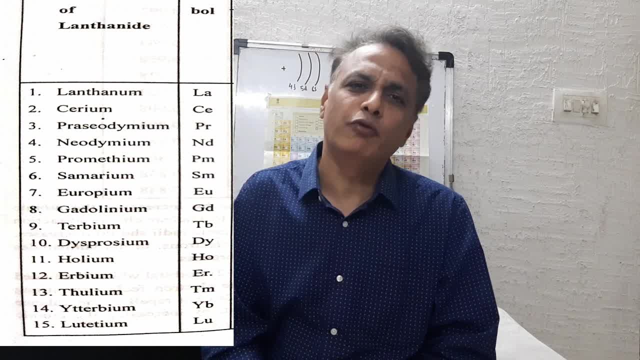 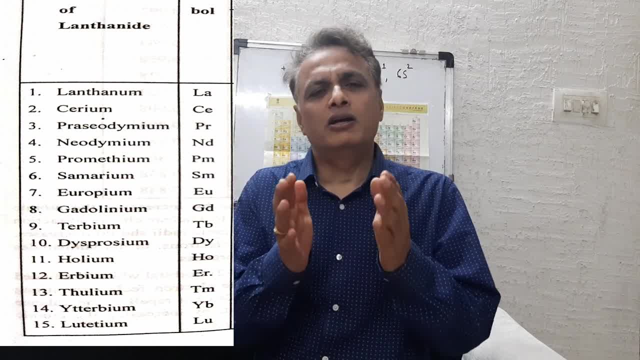 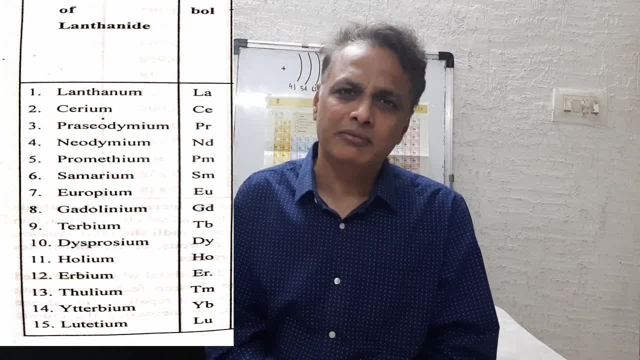 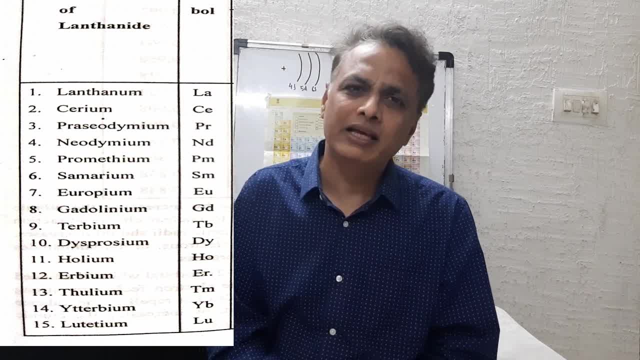 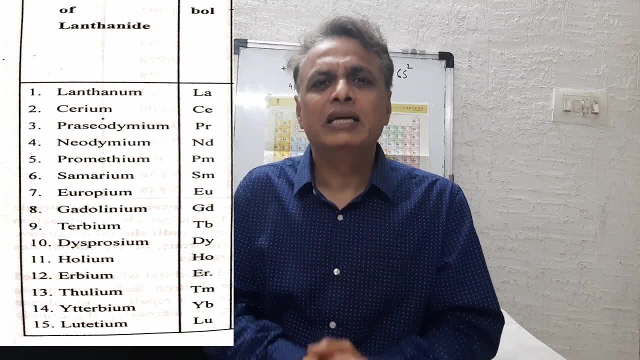 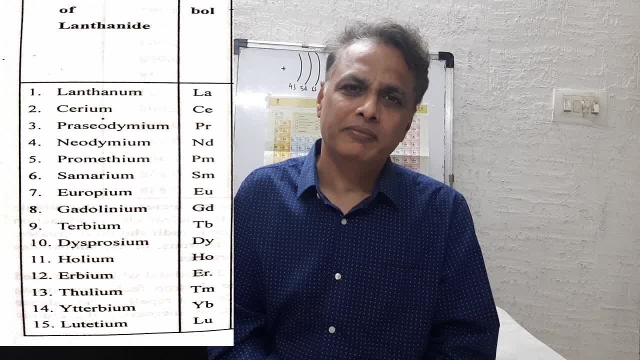 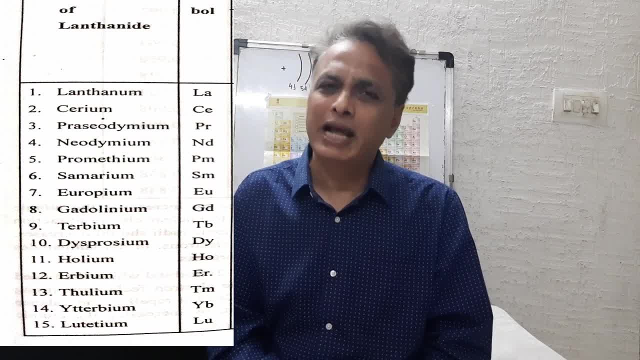 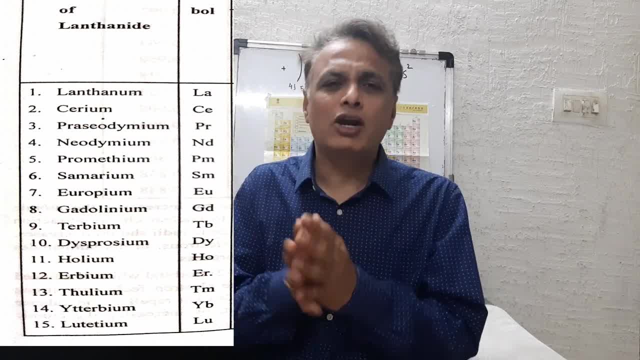 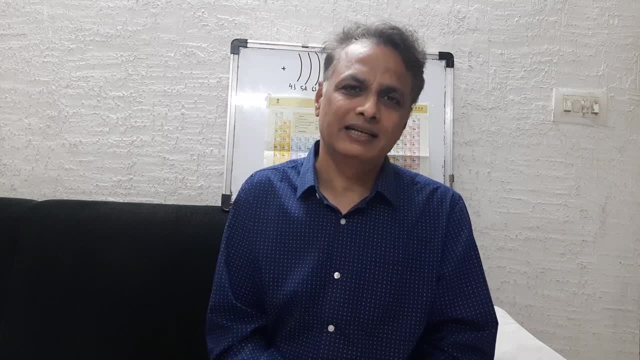 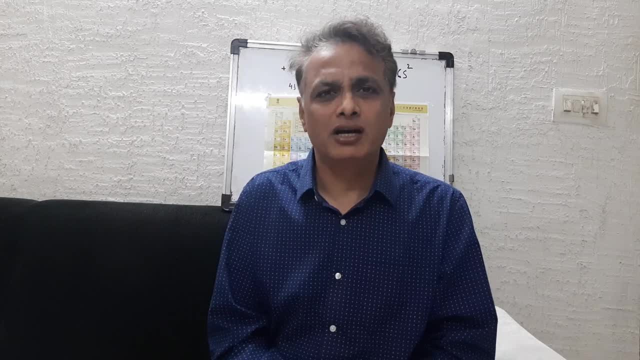 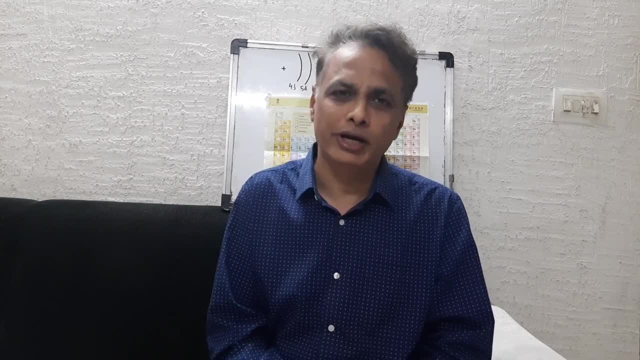 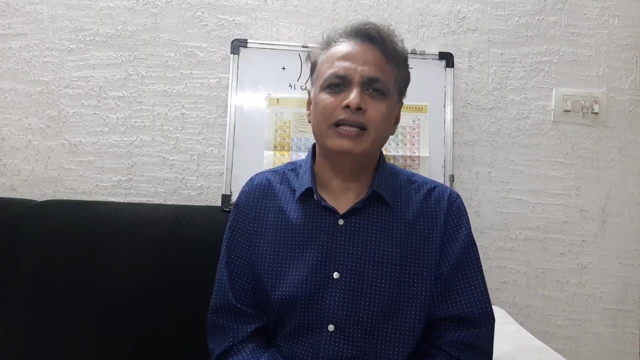 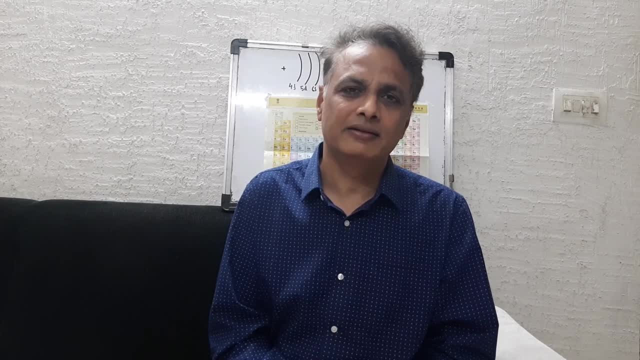 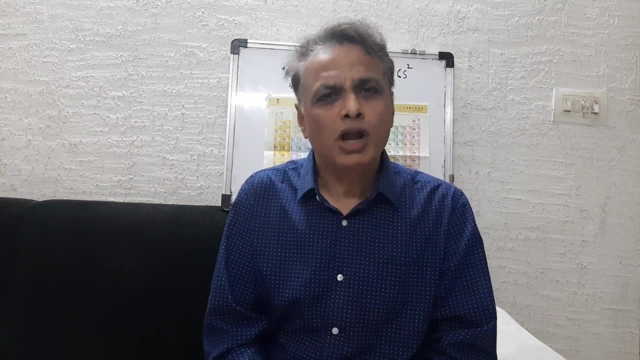 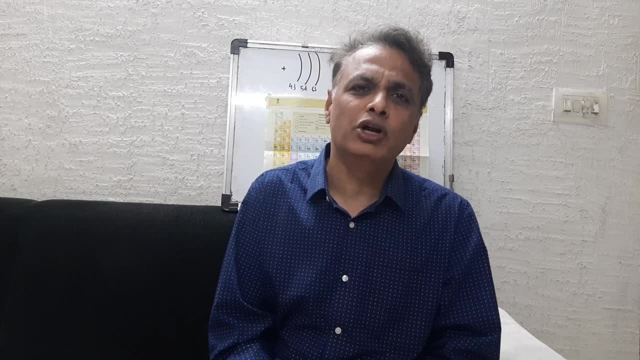 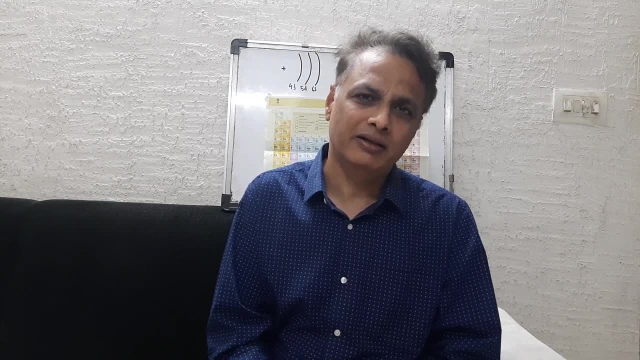 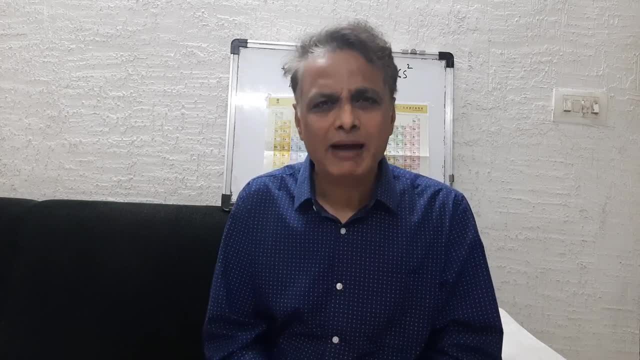 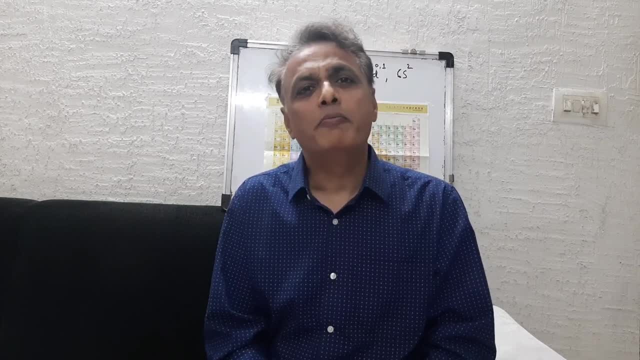 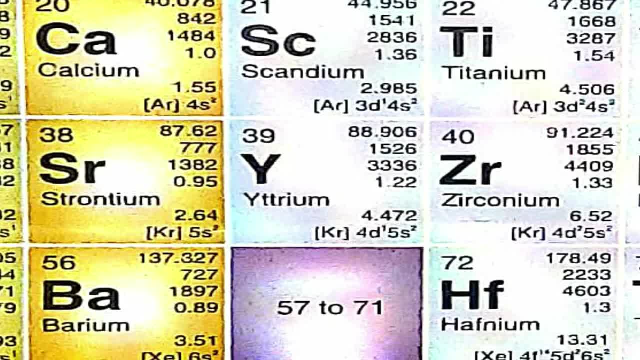 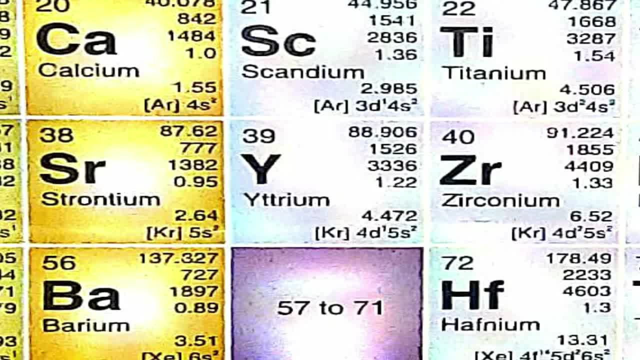 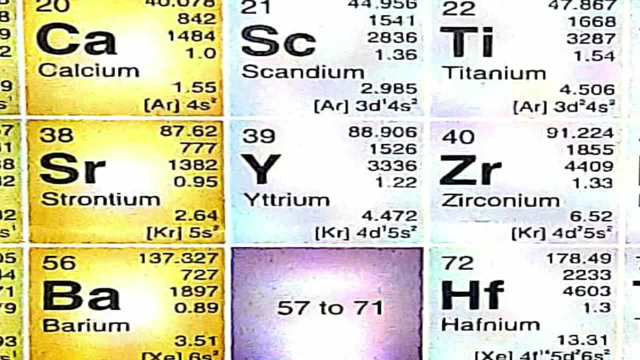 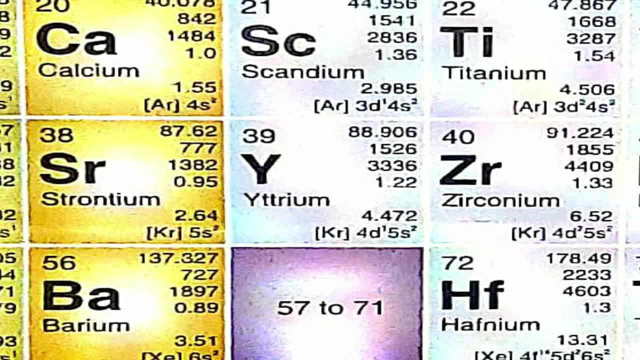 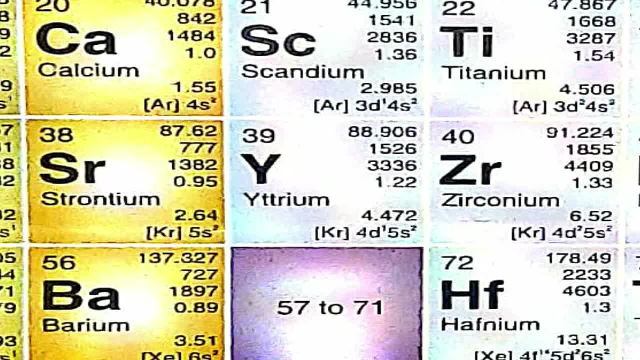 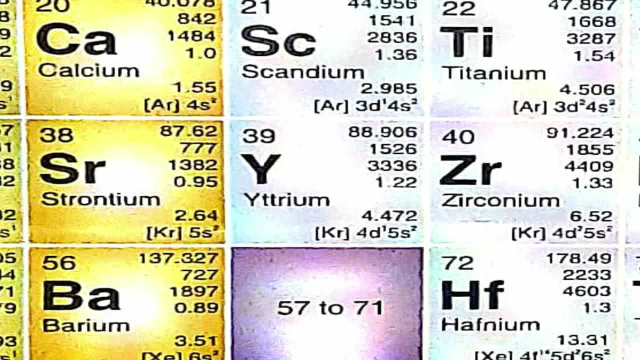 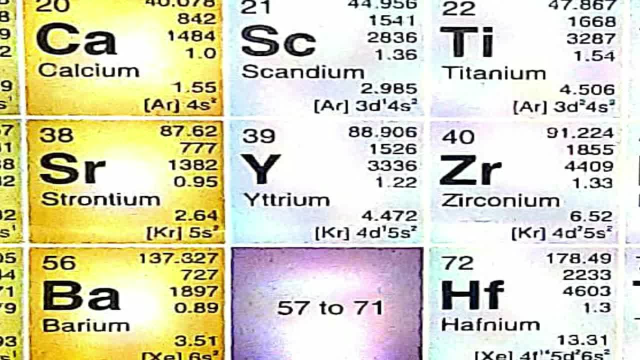 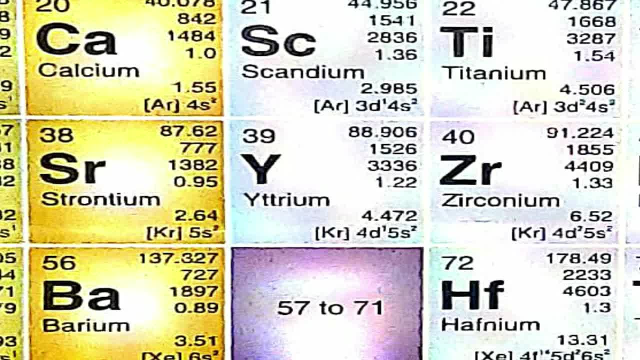 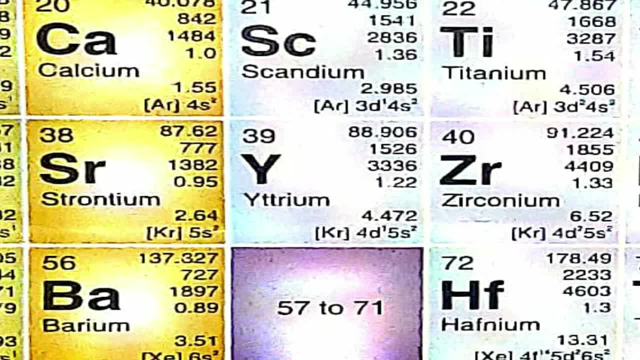 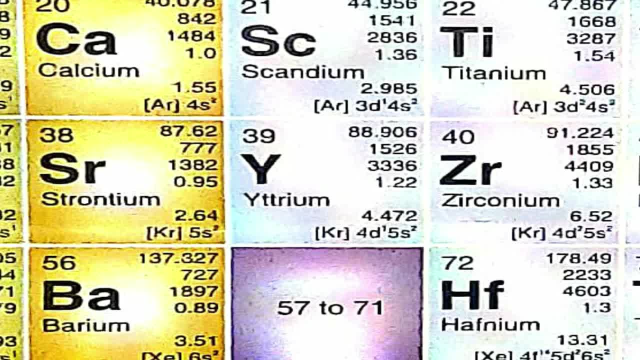 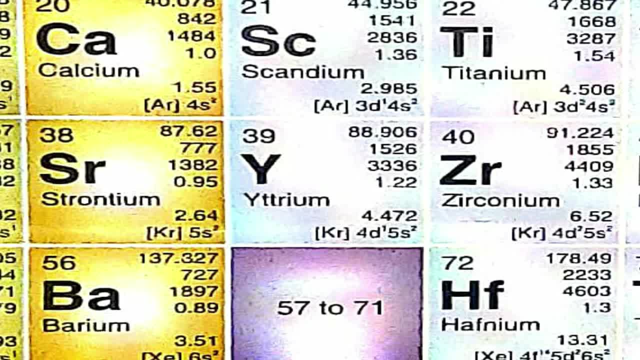 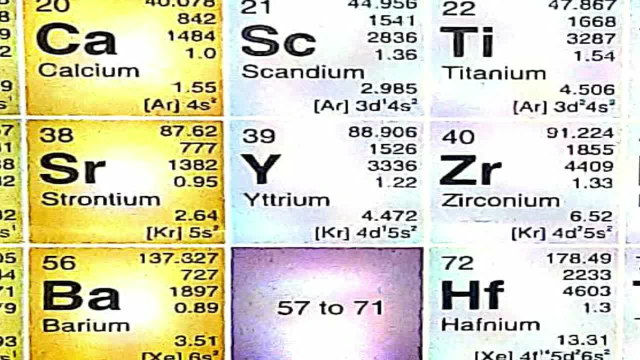 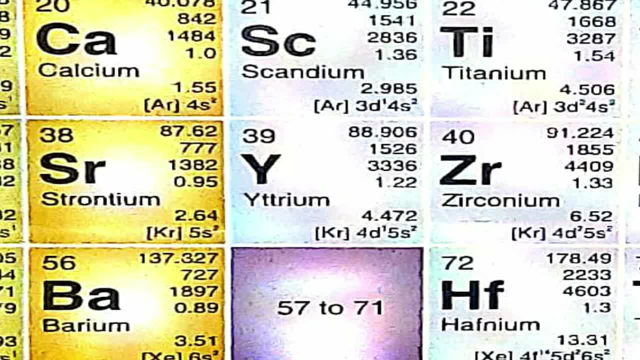 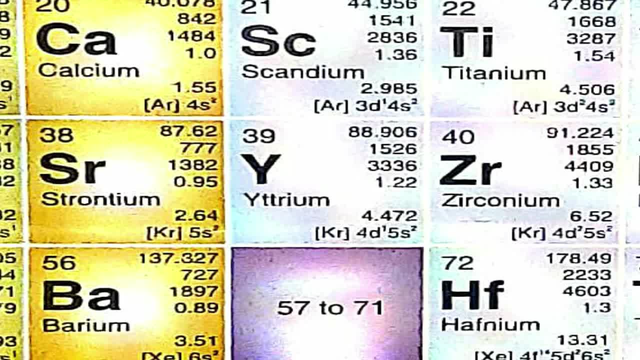 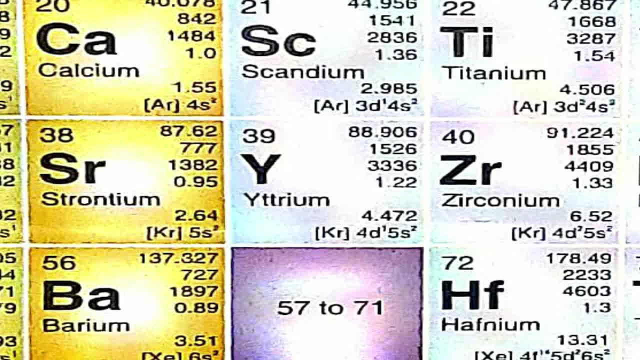 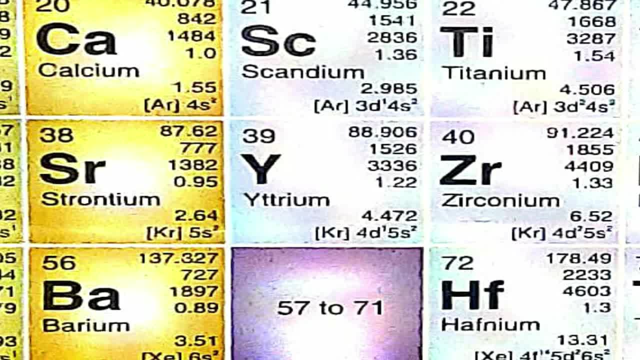 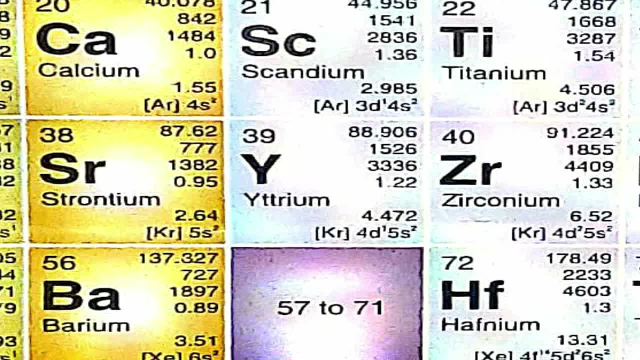 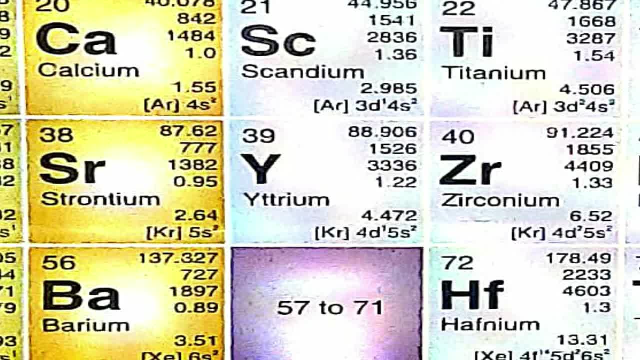 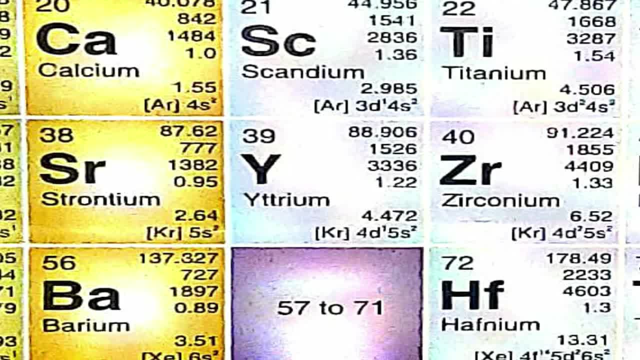 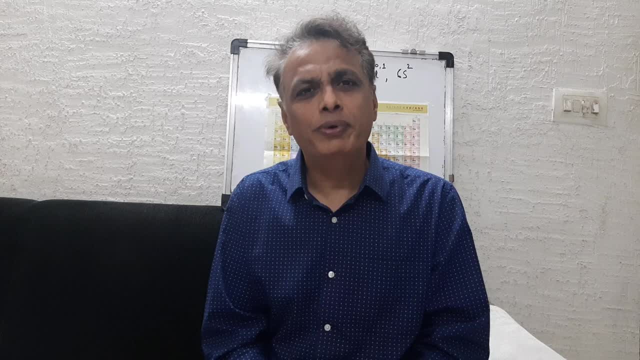 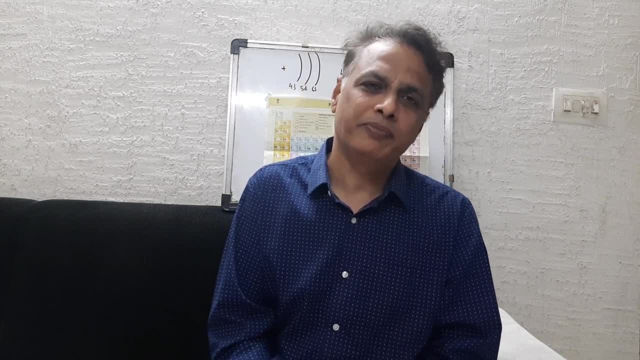 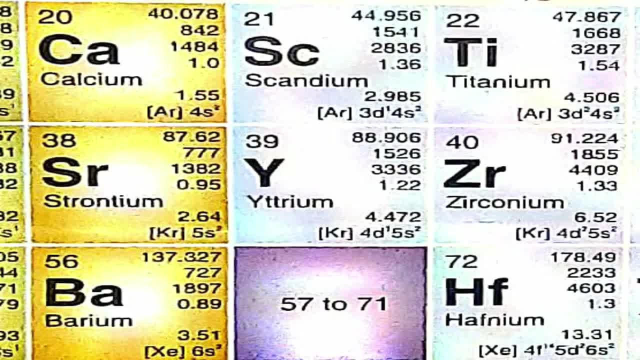 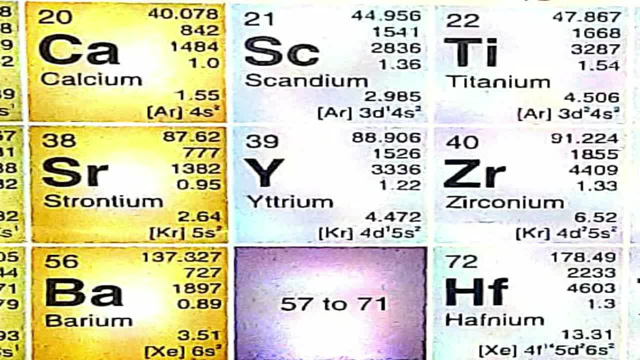 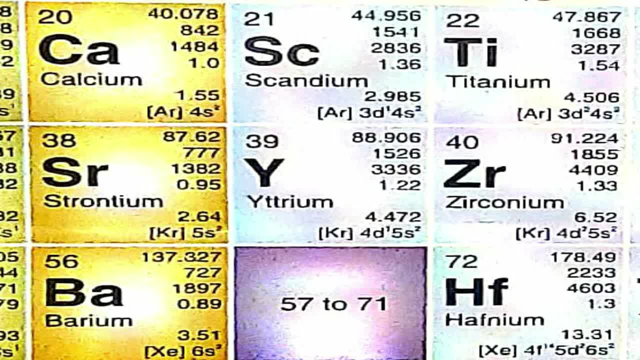 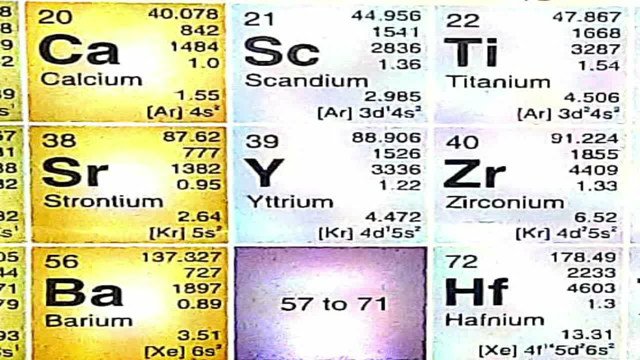 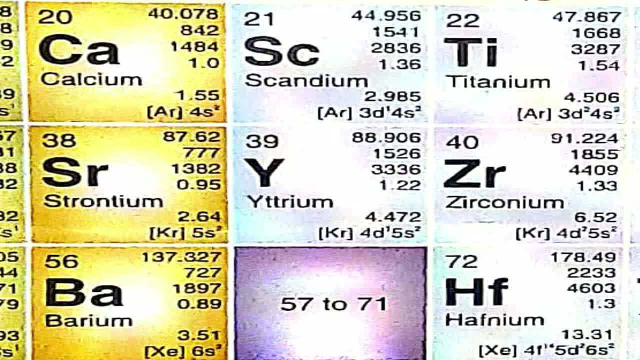 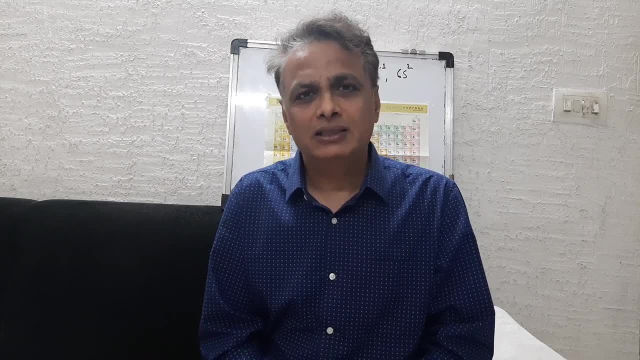 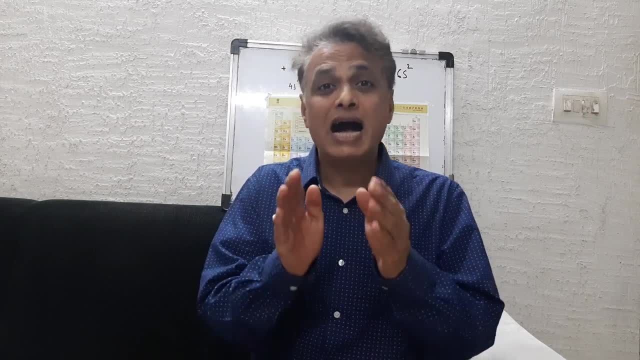 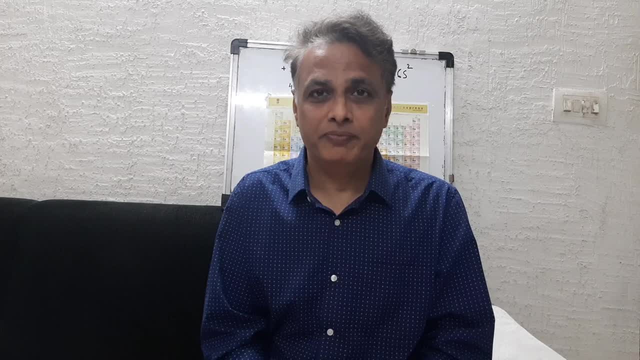 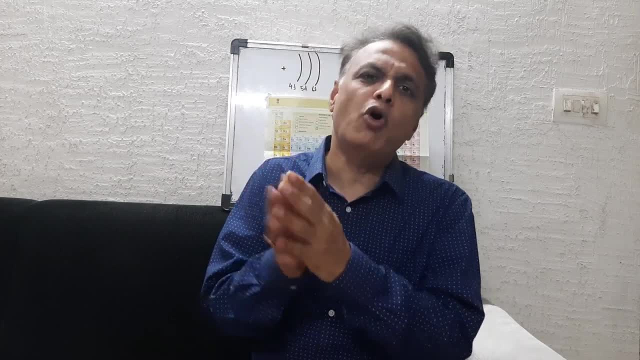 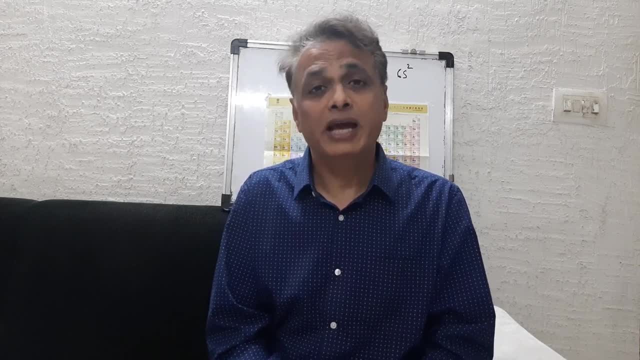 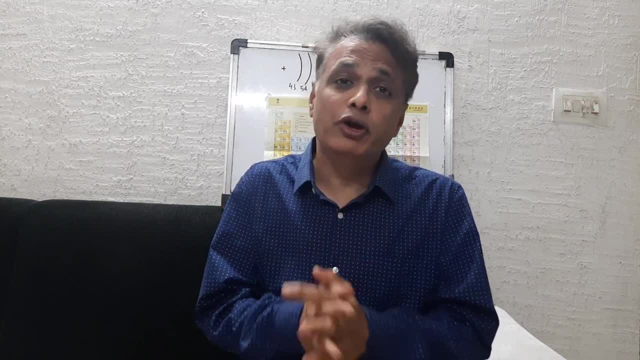 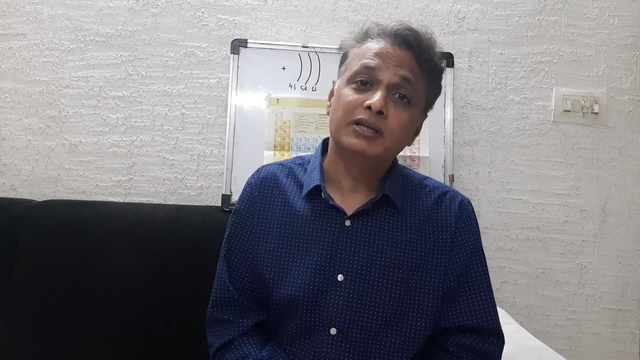 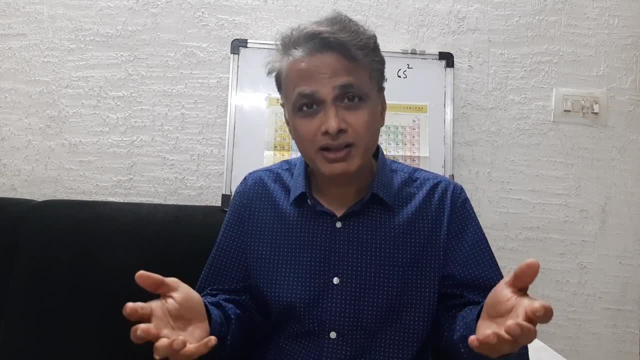 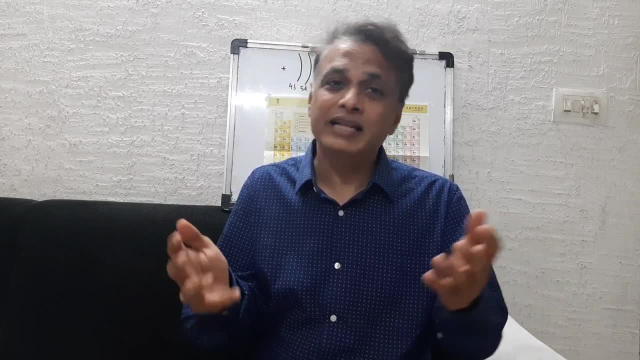 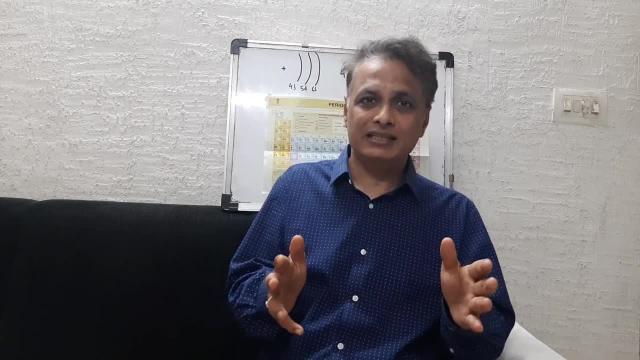